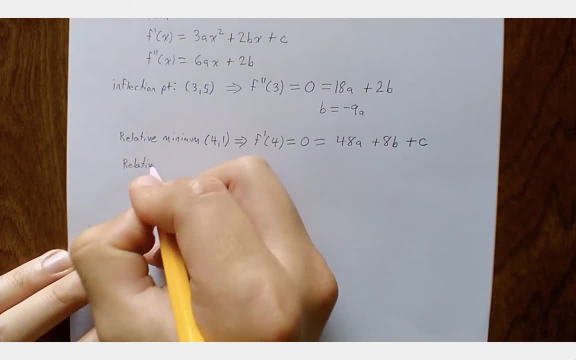 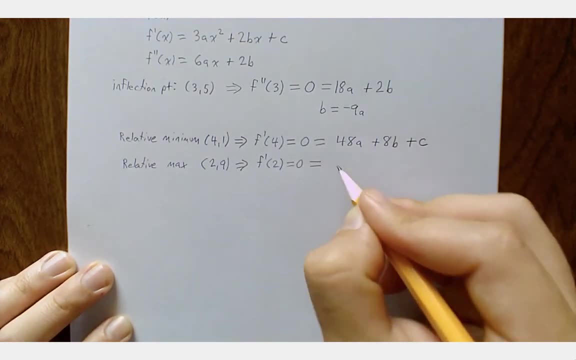 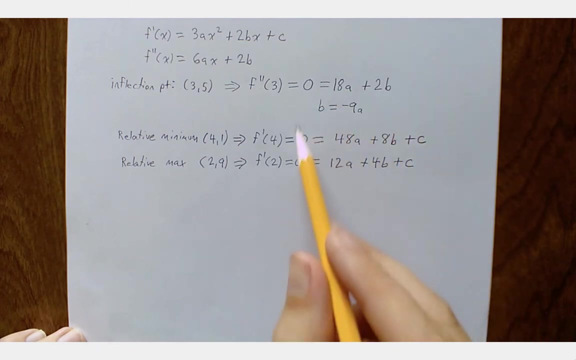 I'll also take the relative max, and the first derivative at 2 is equal to 0.. So now I have three equations and three unknowns, So I'll take this system here and see what I get. In order to do this, I'll take b equal to negative 9a and replace b's. 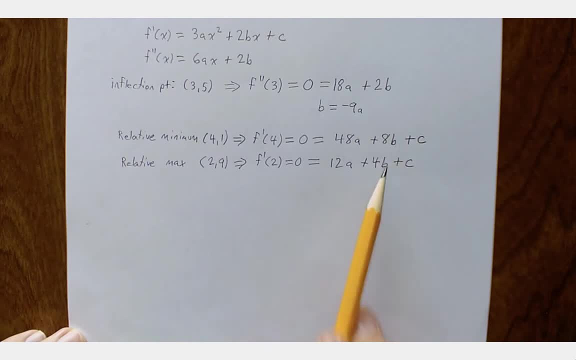 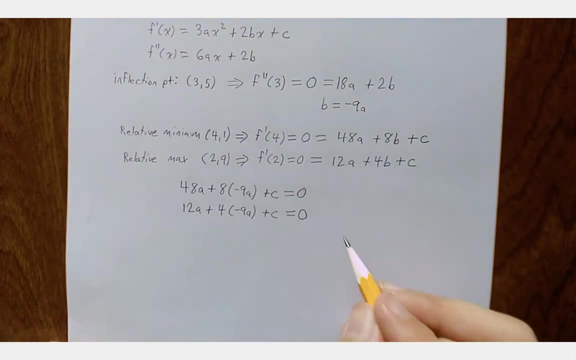 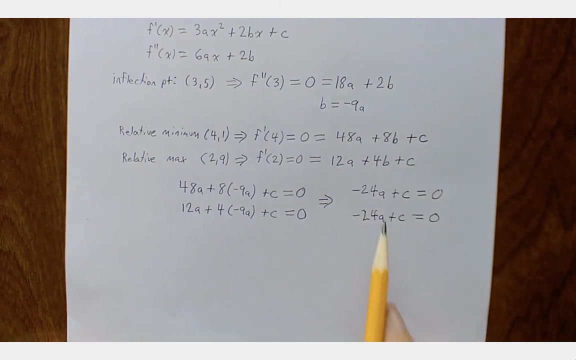 With negative 9a's in these two equations. I'll simplify these And I actually get the same exact equation, so I'll just cross out one of them. There's a little bit of redundancy in this system. Now I'll solve for c and I get that c equals. 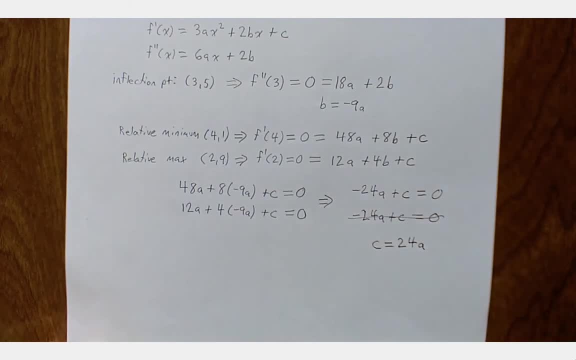 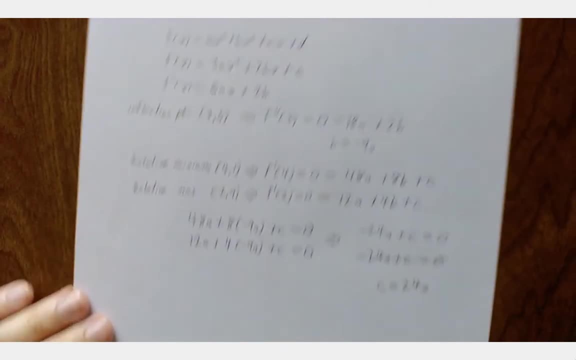 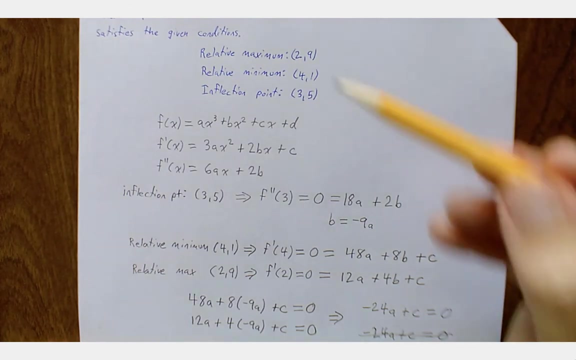 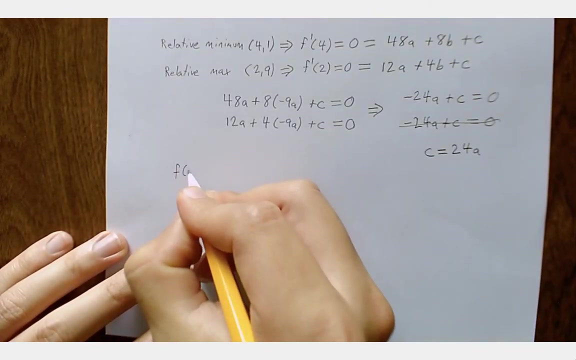 Equals 24 times a. You might be thinking we used all of our conditions, but we have three more conditions, since these points actually lie on the graph, So I'll use just the first point here: 2, 9.. So we know that f of 2.. 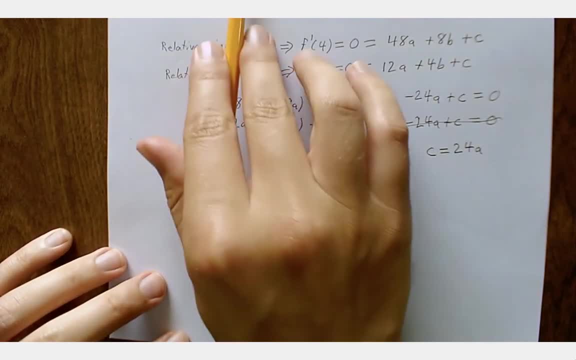 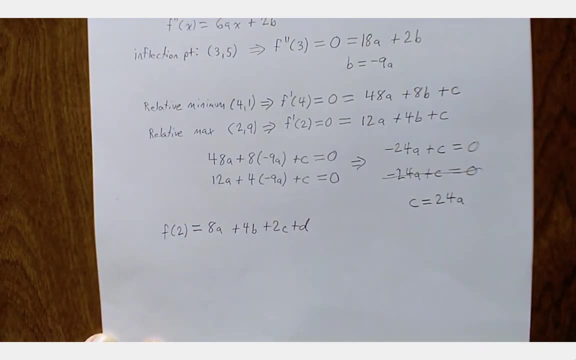 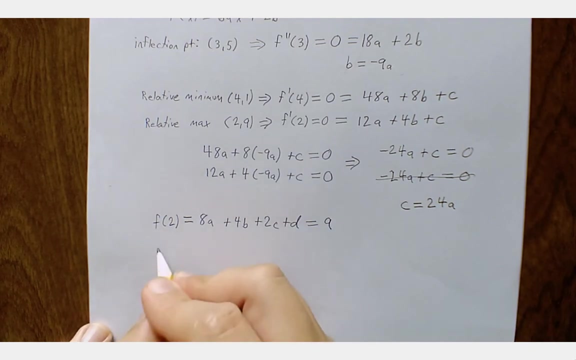 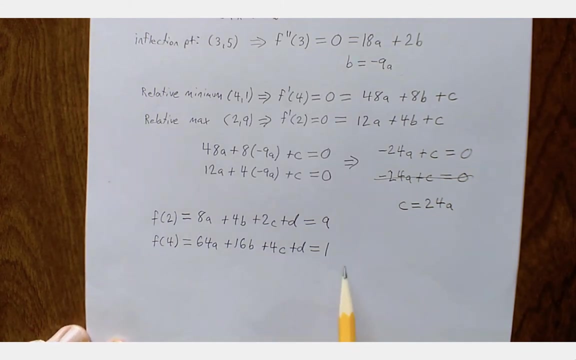 Which when we plug in 2 into Our equation up here, we get this, And that is equal to 9.. I'll take the second point, which is 4, 1, do the same thing. So now I have two equations and I can get c and b in terms of a. 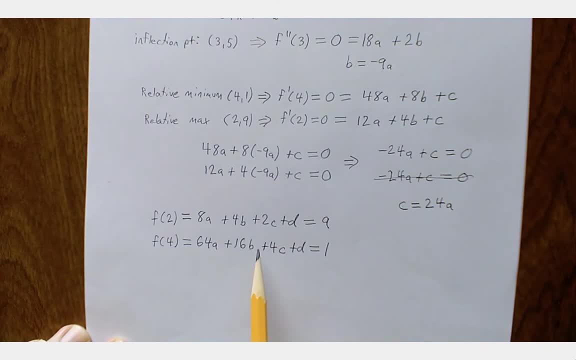 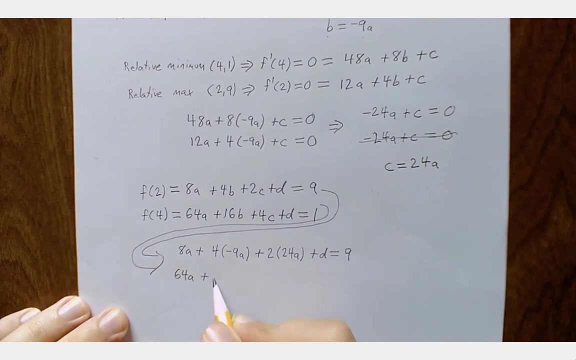 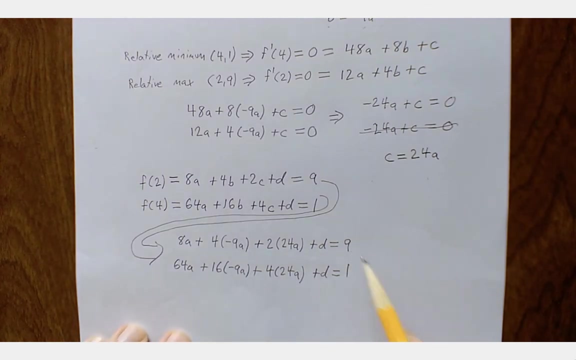 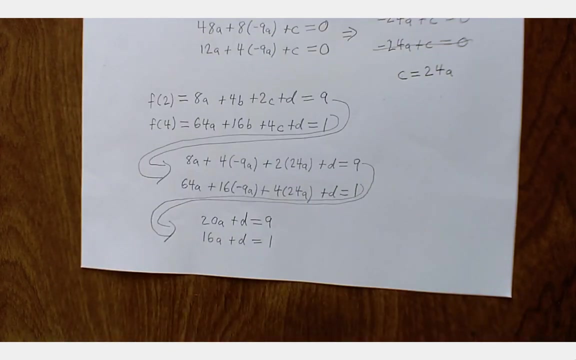 So this will be a system of two equations, equations, two unknowns, which should be solvable. So I'll make those substitutions: b is negative, 9a and c is 24a. I'll simplify both these equations. Now we have a simple system of two equations, two unknowns. I'll subtract the.